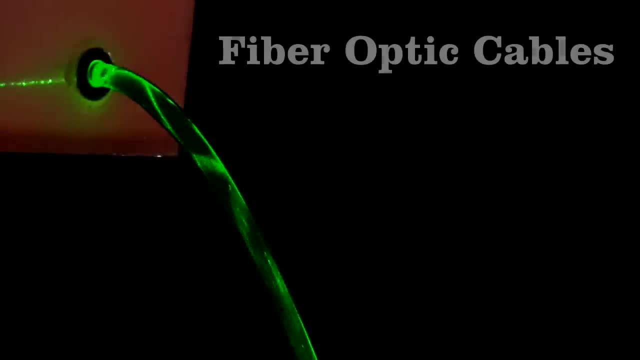 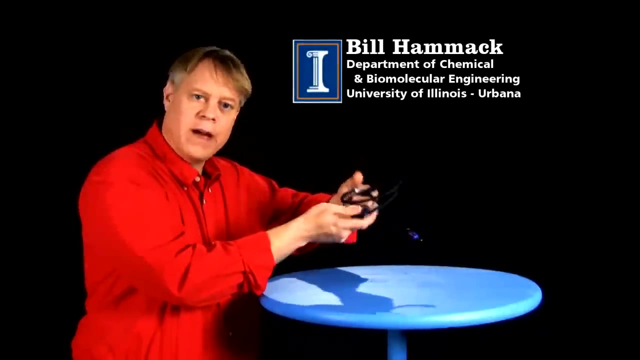 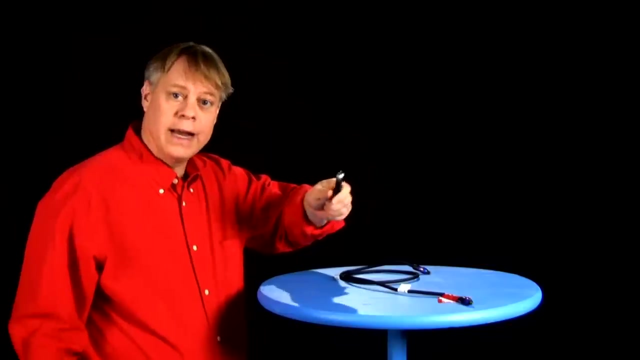 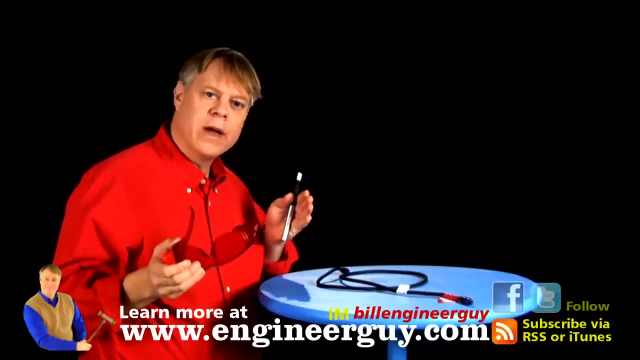 I find this a fascinating object. It's a fiber optic cable for a stereo. If I shine this laser pointer down the cable, it guides the light out the other end. These cables are used to connect our world today and are capable of transmitting information across. 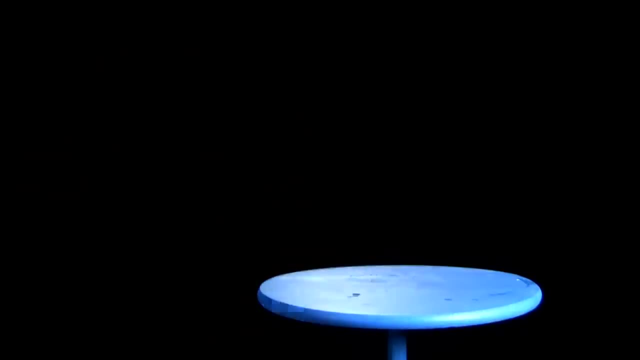 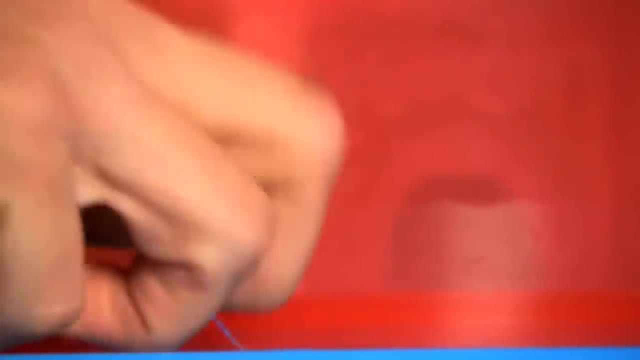 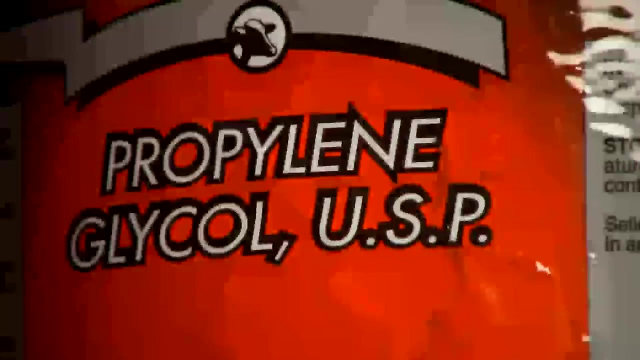 countries and oceans. But first let me show you how it works. I have a bucket that I've modified with a window in front, and on the other side I put a stopper in this hole. right here I have a bottle of propylene glycol with just a little bit of creamer in it. a 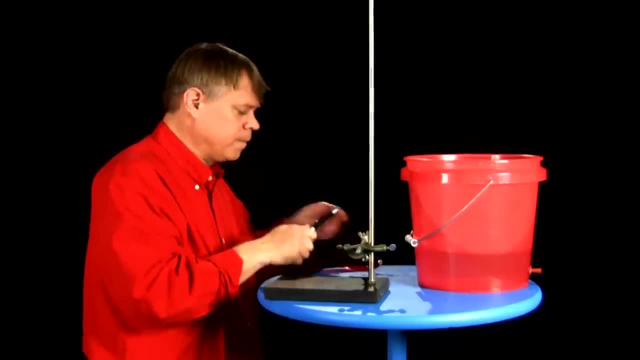 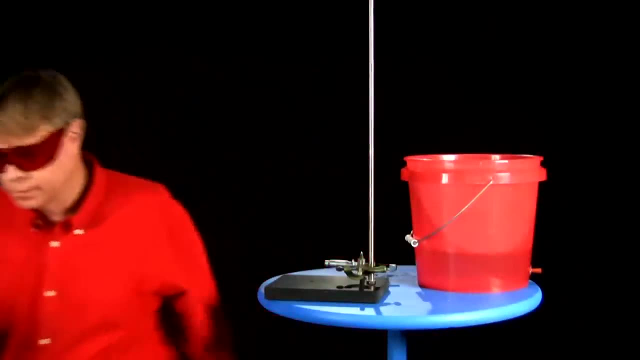 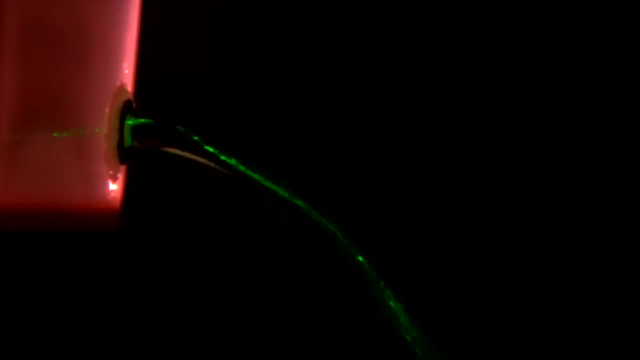 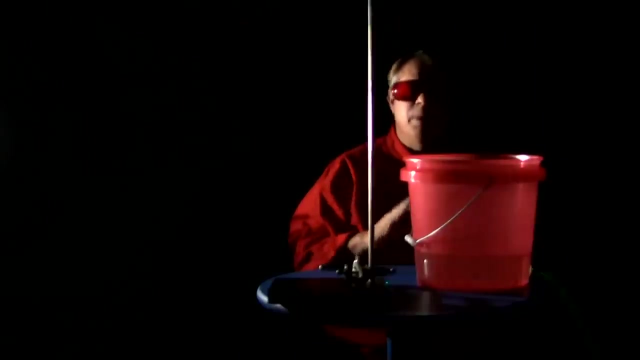 ring stand and, of course, a laser pointer. Now keep your eye on this plug when I turn off the lights. That's wonderful. The light follows the liquid flow all the way to the bucket. Amazing, It does this because of total internal reflection. As the light enters the stream, it is reflected as soon as it hits. 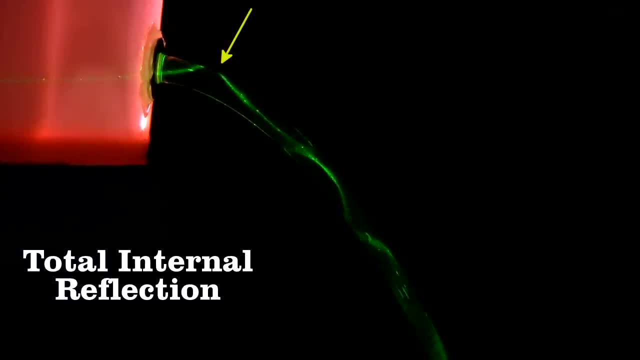 the interface between air and liquid. You can see here the first reflection and then the second and the third. This occurs because there's a difference between the index of refraction of the guide material- here propylene glycol- and the outside air, in this case. 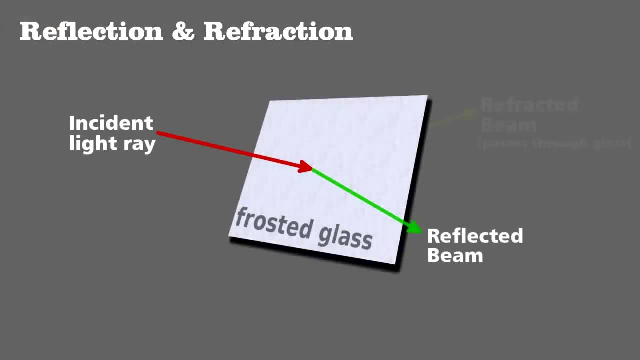 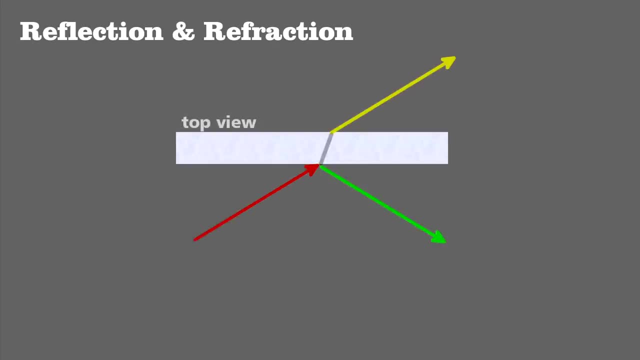 Recall that any time light strikes a surface, it can either be absorbed by the material reflected from it or pass into and through it. the latter we call refraction. It's easier to see from a top view. Reflection and refraction can happen at the same time. but if a light 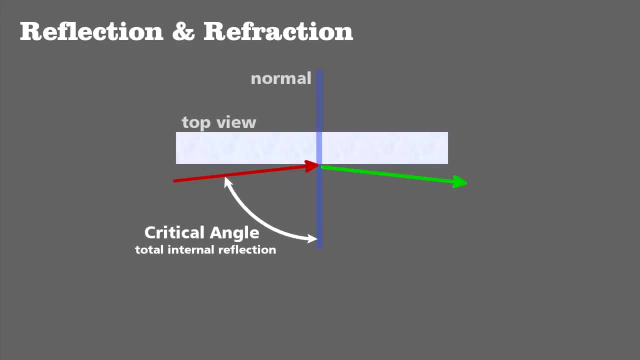 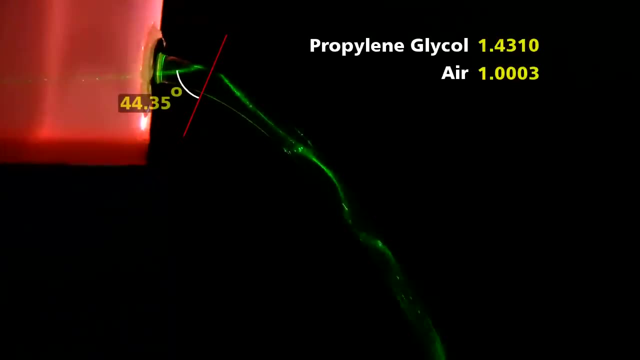 ray hits the surface at an angle greater than the critical angle, it will be completely reflected and not refracted. For this, propylene glycol and air are the same As long as a beam hits the surface at an angle greater than 44.35 degrees, measured from. 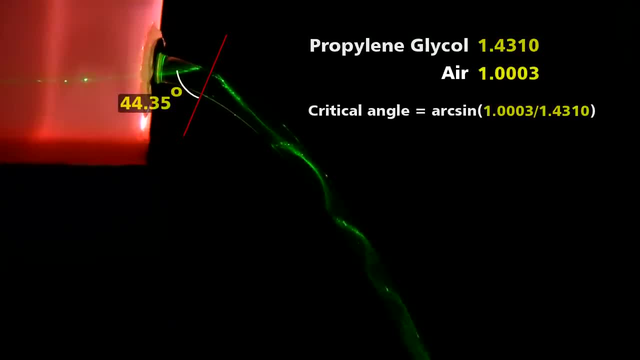 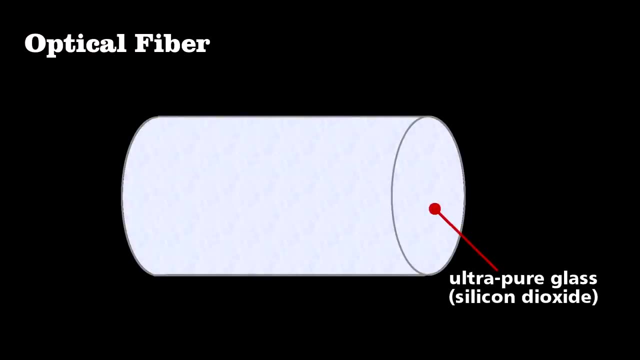 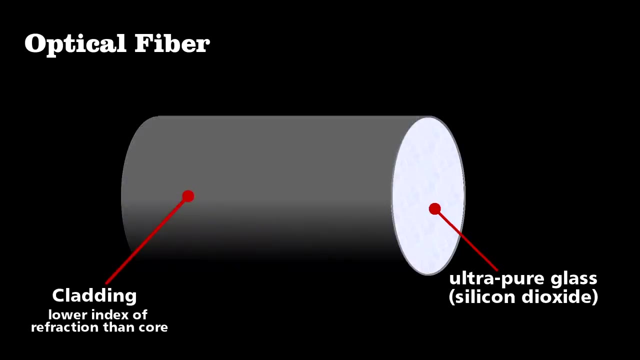 the normal, it will propagate down the stream via total internal reflection. To create this same effect in an optical fiber, engineers create a core of glass, usually pure silicon dioxide, and an outside layer called cladding, which they also typically make from silicon dioxide, but with bits of boron or germanium to decrease its index of. 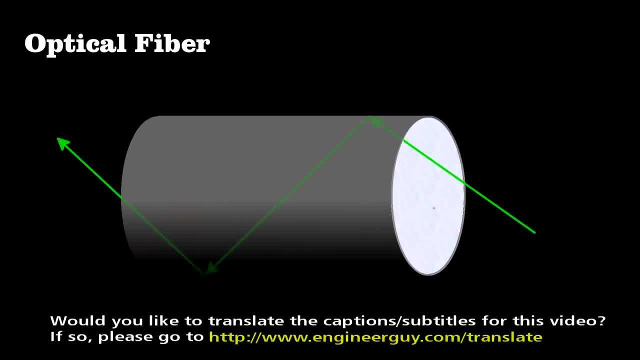 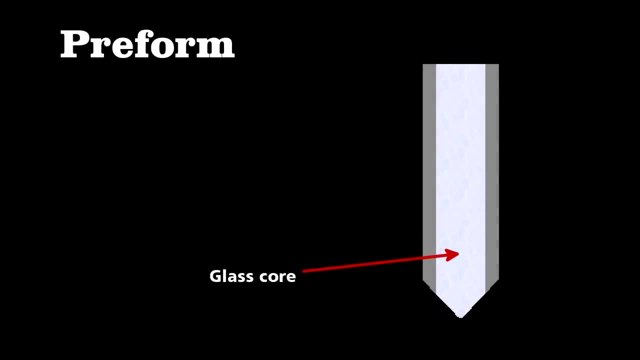 refraction. A one percent difference is enough to make a fiber work, To make such a long, thin piece of glass. engineers heat a large glass preform. Its center is the pure core glass and the outside the cladding. They then draw or pull a fiber by winding the melt onto. 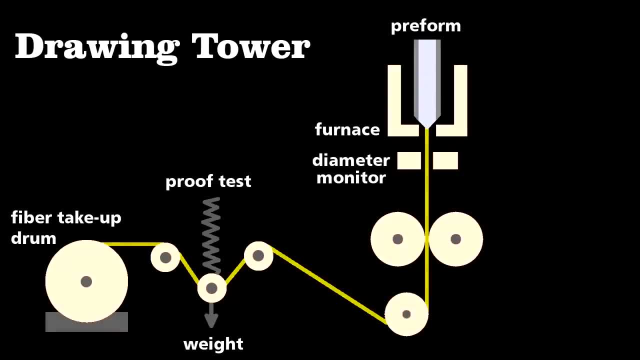 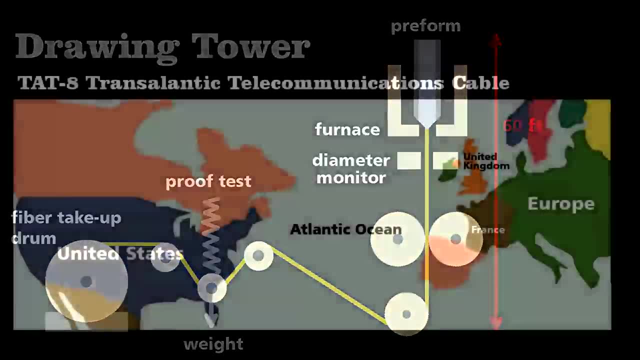 a wheel at speeds up to 1,600 meters per second. Typically, these drawing towers are several stories tall. The height allows the fiber to cool before being wound onto a drum. One of the greatest engineering achievements was the first ocean-spanning fiber-optic cable. 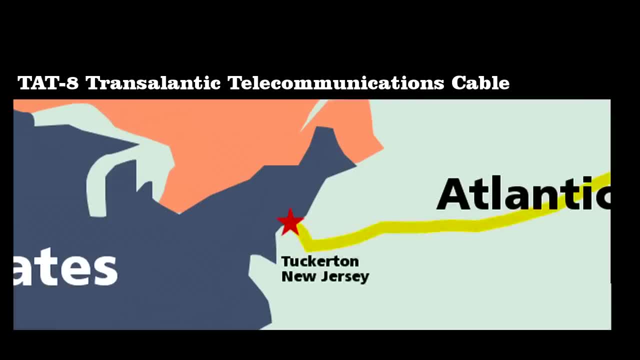 Called TAT-8,. it extended from Tuckerton, New Jersey, following the ocean floor, over 35,000 miles. The fiber was then transferred to the ocean floor, which was the first fiber-optic cable in the world. TAT-8 is the largest fiber-optic cable in the world. It is the largest fiber-optic fiber-optic. 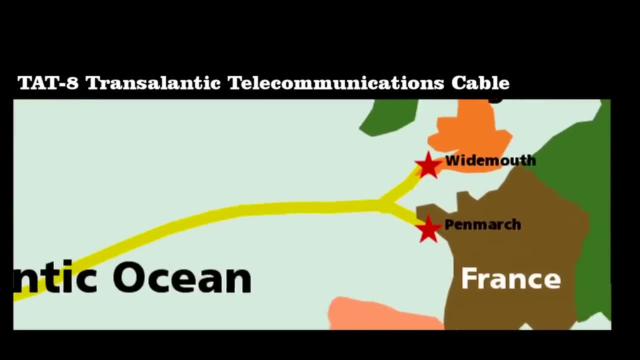 cable in the world. It was used in the war from 146th to 146th. The cable has been used on the ocean floor over 3,500 miles until branching out to Whitmouth, England, and Palmash, France. Engineers designed the cable carefully to survive on the ocean floor At its center. 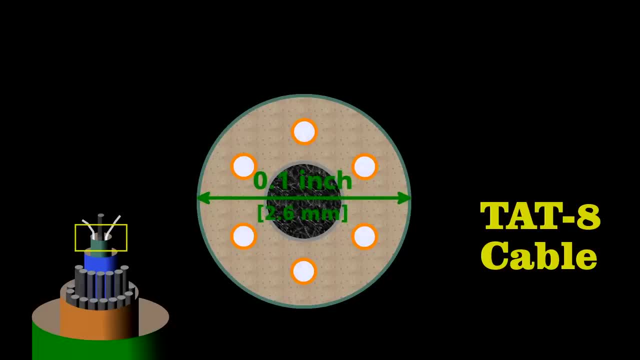 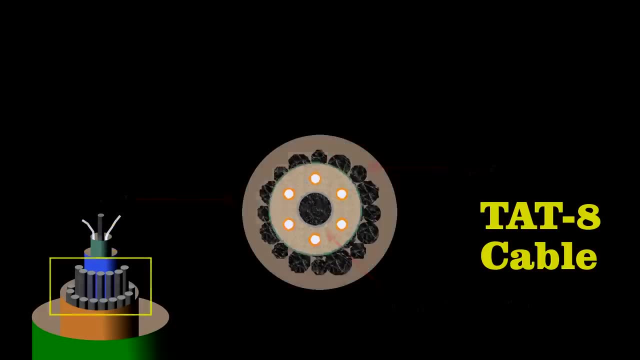 lies the core, Less than a tenth of an inch in diameter. it contains 6 optical fibers wrapped around a central steel wire. They embedded this in an elastomer to cushion the fibers, surrounded it with steel strands and then sealed it inside a copper cylinder. 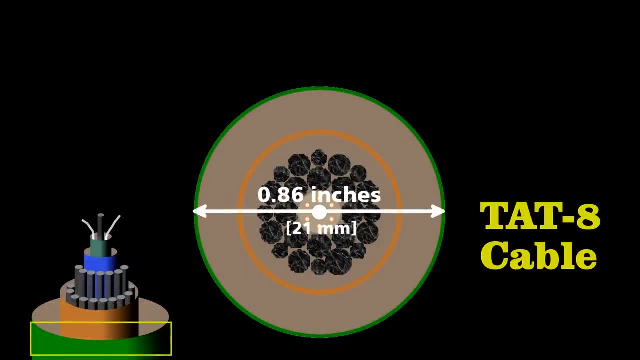 to protect it from water. The final cable was less than an inch in diameter, yet it could handle some 40,000 tons of fiber thousand simultaneous phone calls. The essence of how they send information through a fiber optic cable is very simple. I could have a prearranged signal with someone at the other end, Perhaps. 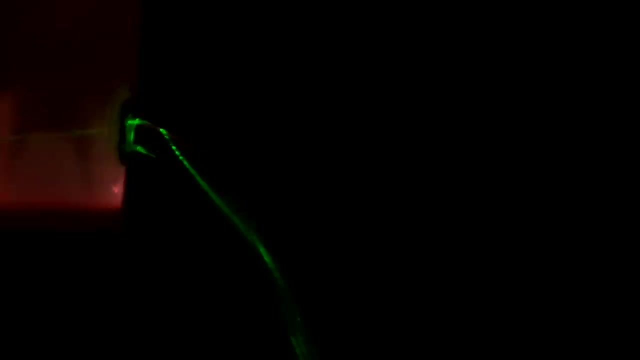 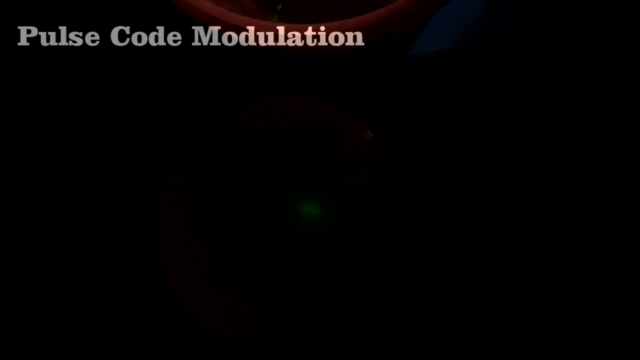 we'll use Morse code and I just block the laser so that the person at that end sees flashes that communicate a message. To transmit an analog signal, like voice, from a phone call along the cable, engineers use pulse code modulation. We take an analog signal and cut it up into sections. 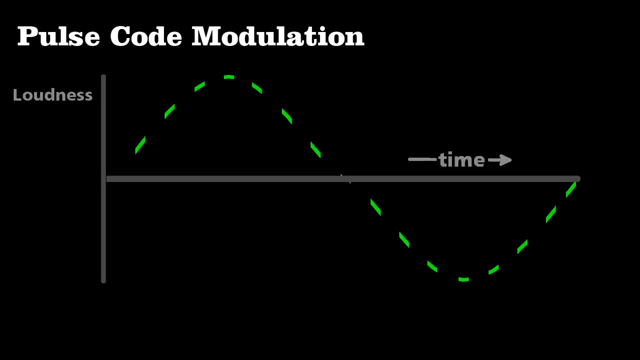 and then approximate the wave's loudness or amplitude as best we can. We want to make this a digital signal, which means discrete values of loudness and not just any value. For example, I'll use four bits, which means I have 16 possible values for the loudness. So the first four. 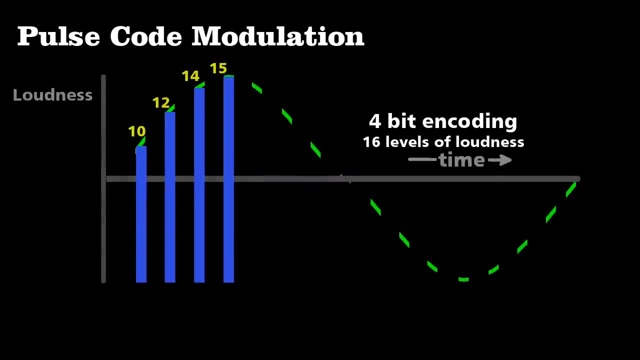 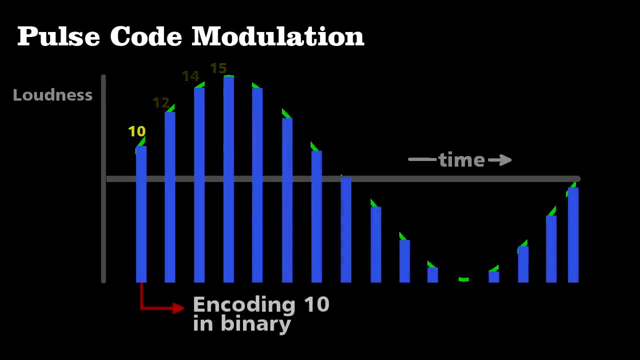 sections of the signal could be approximated by about 10,, 12,, 14, and 15.. We then take each section and convert its amplitude to a series of ones and zeros. The first bar of value, 10, when encoded.